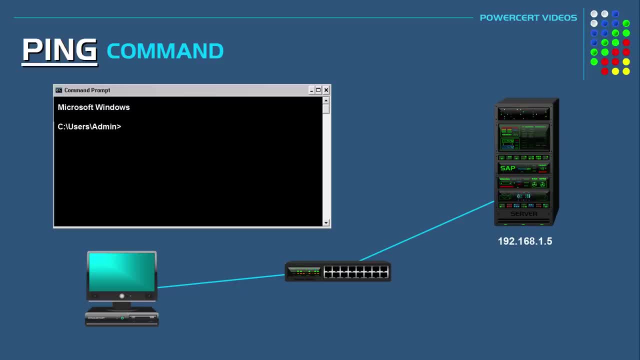 local area network. So we would open up a command prompt and then we would type the word ping along with the IP address of the server and then press enter. Then the ping utility will send out four data packets to the IP address of the server. Then our computer will wait for a response. 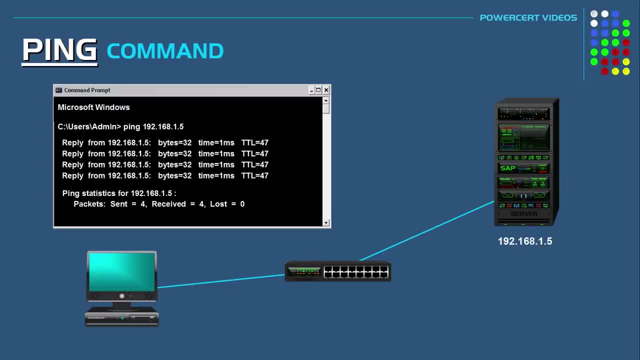 Then the server will send the data packets back to us as a reply, And these replies are called echo reply requests And these replies inform you about what's happening with the server we pinged. So, for example, if we received a reply, then that is a good sign. 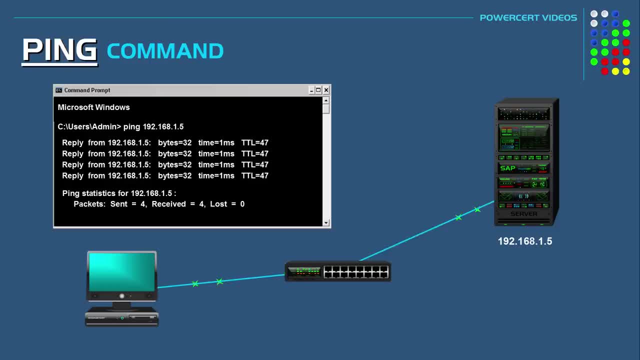 Then that means that there is network connectivity between us and the server, Whether that server is on your local area network or over the internet. So four packets were sent and then four packets were received. But if we pinged the same server and this time if we didn't get a reply, then that 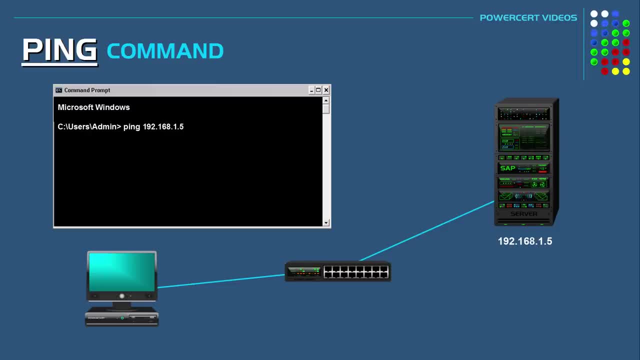 means that the server didn't reply back, And it could mean that there is no reply. There is no network connectivity between our computer and the server. Now, this could be for several different reasons. So, for example, when we ping the server and if we get a message back that says request. 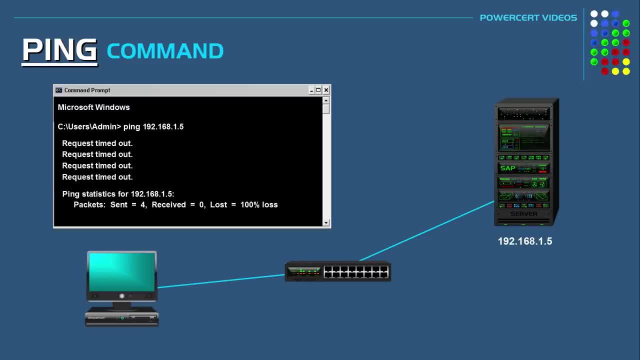 timed out, Then that could mean that the server is powered down. Or it could also mean that the server is up and running but it's using a firewall that's blocking all ping requests. Now what happens when you use a server that's on your computer and the server is on your network? 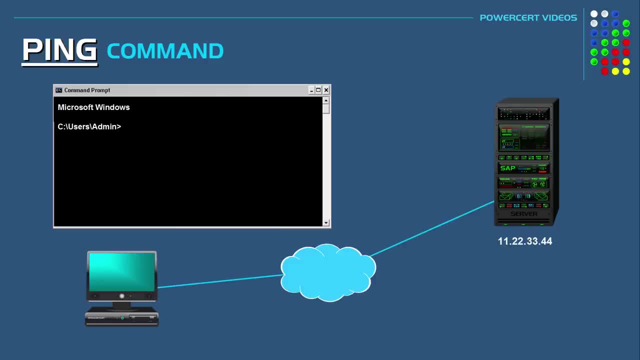 you try and ping a host and not all of the data packets reply back to you. So, for example, when you ping a host, your computer sends out four data packets, but sometimes you may only get one, two or three packets back instead of the four that you sent out. Well, this is called packet loss. 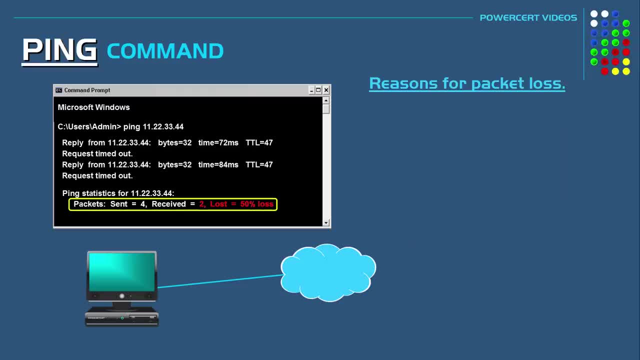 and packet loss can occur for several reasons. It could mean that there's network congestion- If there is a lot of traffic on a network and the network can't handle all that extra traffic, then data packets will get dropped. Or it could also happen because of faulty hardware. 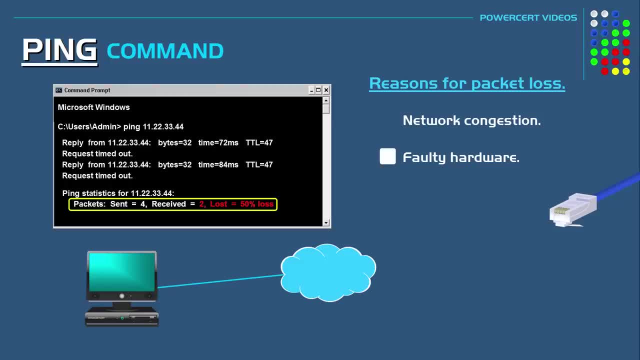 such as bad cables or bad wiring, Or it could be a bad network card or bad connections, Or it could be a bad modem, which is exactly what happened to me in my case A few years ago. I was constantly lagging in just about everything I did on the internet. 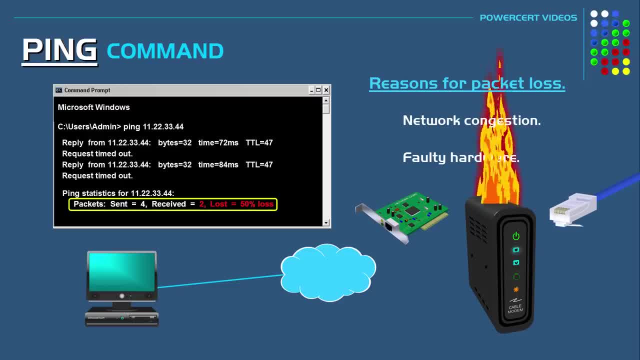 So I didn't have a lot of data and I didn't have a lot of data. So I didn't have a lot of data. I did a continuous ping test and I was dropping at least one-third of my packets fairly consistently. So I determined that it had to be my modem. So I had it replaced and it solved the. 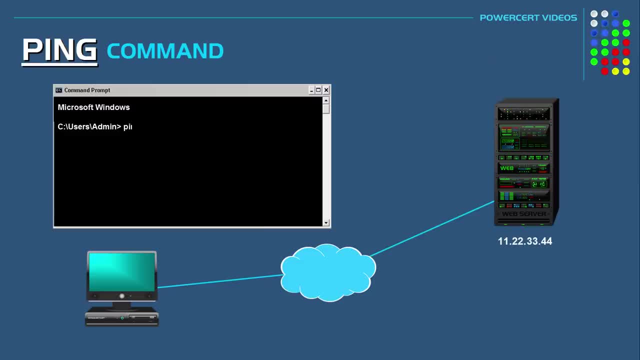 problem. Or, in another scenario, if we wanted to ping a remote server on the internet and if we got a message that says destination host unreachable, then that means that a route to the destination doesn't have any information on how to route data to the destination, Or it could also 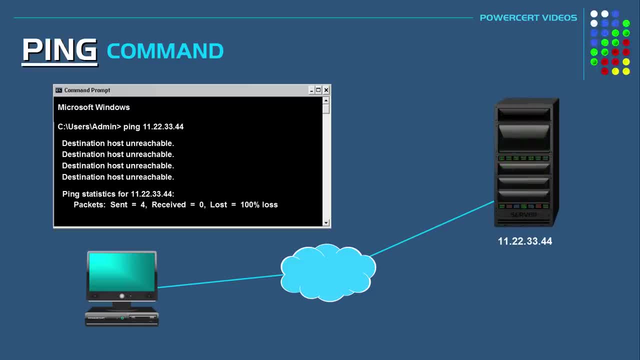 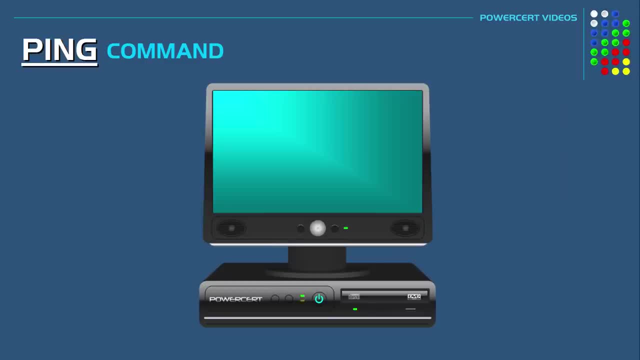 mean that the remote server is down or disconnected from the network, Or it could also mean that your computer is not connected to a network, So let's use the ping command in a typical scenario. So suppose someone tells me that they don't have an internet connection because they can't access. 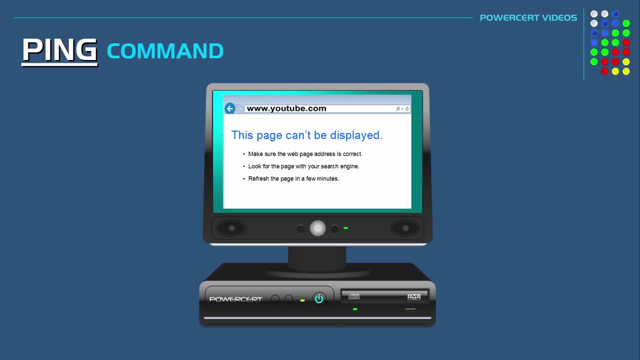 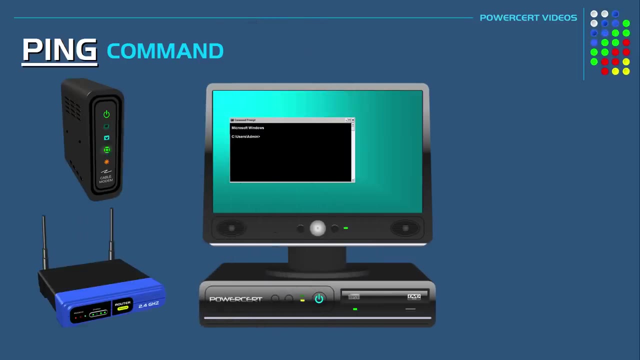 any web pages with their computer, which is a pretty common issue. So the first thing I do is that I would sit at their computer and use the ping utility to see if in fact, they are not connected to the internet. So even before I check their modem or router or any cable, 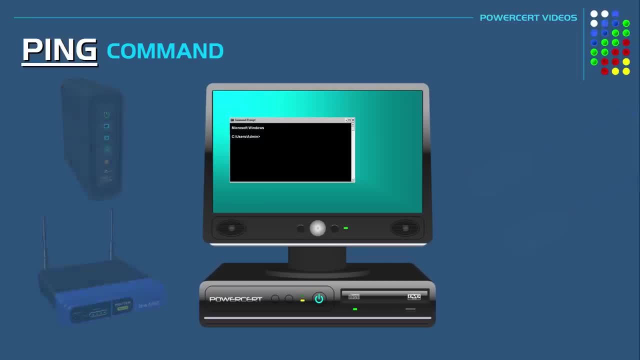 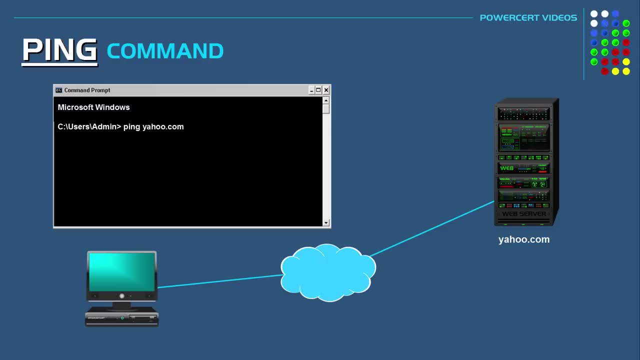 connections. the first thing I do is do a simple ping test. So I would open up a command prompt and see if I can ping a website such as yahoocom. Now notice, in this method I'm actually pinging the domain name yahoocom. and now I'm going to ping the domain name yahoocom. and now I'm going to. 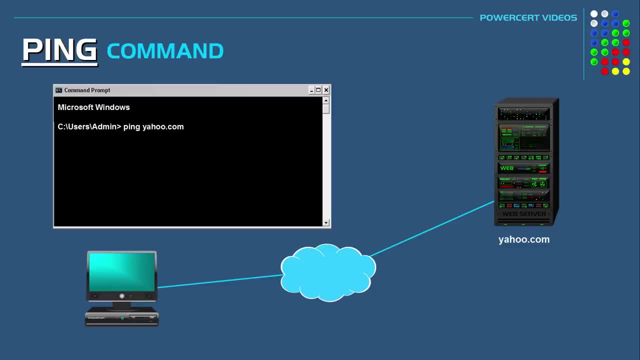 ping the domain name yahoocom, But I'm really going to be using the domain name yahoocom and not its IP address, Because by doing it this way, I'm also testing name resolution, issues related to DNS And also, besides that, I don't have Yahoo's IP address memorized. So by pinging yahoocom, 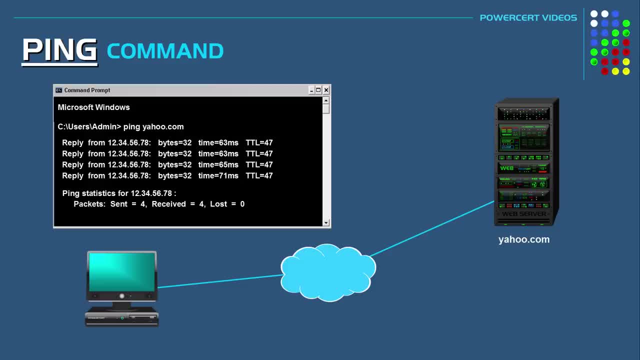 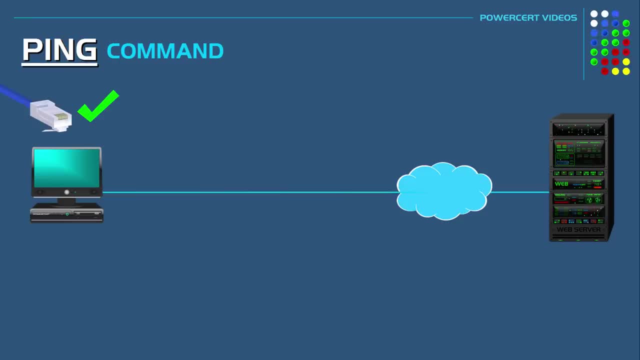 and if the ping is successful, then I know that we are connected to the internet, Because when I got a successful reply from yahoocom, then I automatically know that all of my hardware, such as my cable, the network card, the router and the modem, are all working correctly, including my internet service. 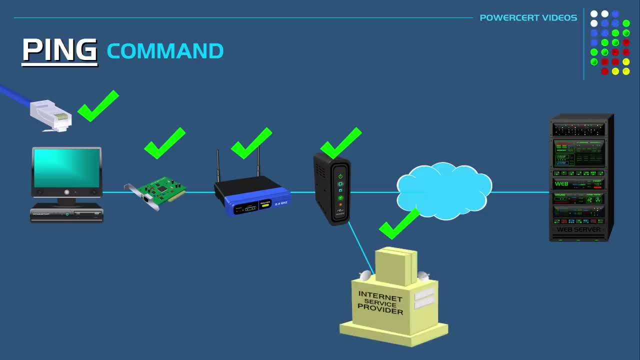 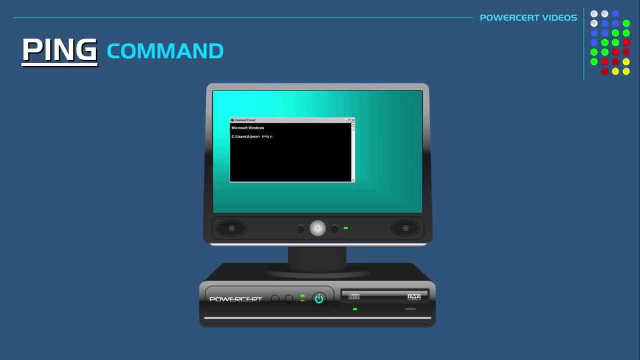 provider. So now I know that the reason that this computer can't bring up web pages is related to software and not hardware. So the problem is most likely with their internet browser or it's a firewall issue. So by doing a ping test first, it saved me a lot of time because I bypassed the 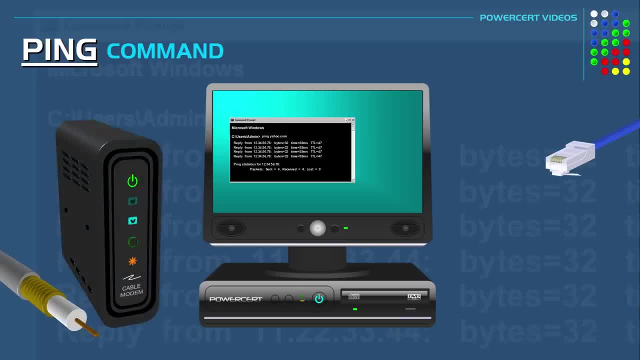 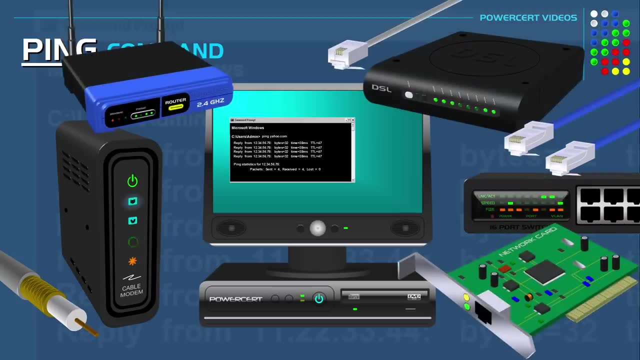 hassle of looking around for the modem or the router, or looking at LEDs or checking the cables, or looking behind the computer to see if the network cable is plugged into my network card. I simply sat down and did a simple ping test. So really the only time you need to check your 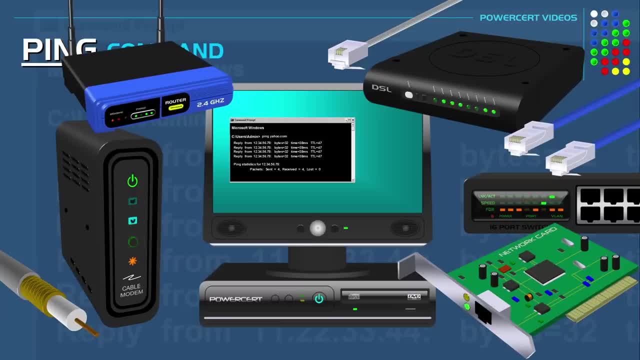 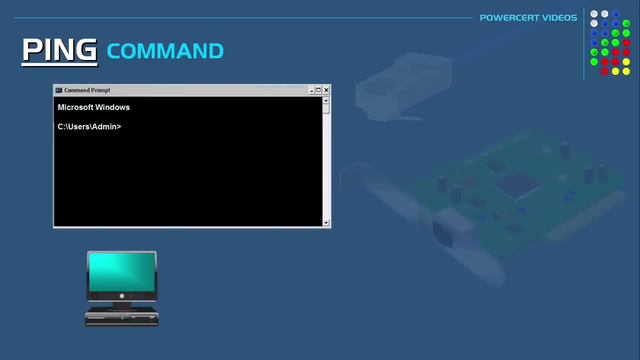 hardware is if the ping was not successful. However, even before you start checking hardware, you can also use the ping command to check other things, such as testing if your network interface card is working correctly or not. If your network interface card is not working correctly, you can. 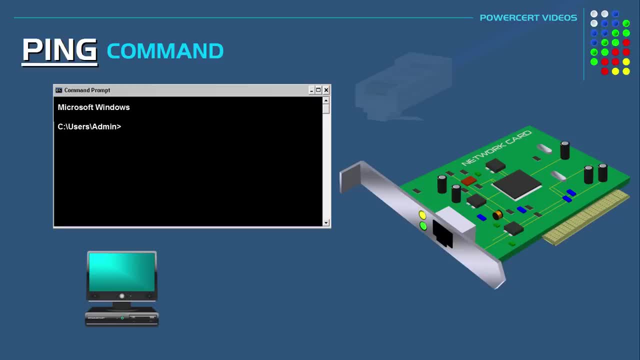 use a loopback test. A loopback test will send out signals back to your computer for testing purposes. So at a command prompt I would type ping and then the loopback IP address, which is 127.0.0.1, or you can simply type ping localhost, which does the same thing. And if the ping was? 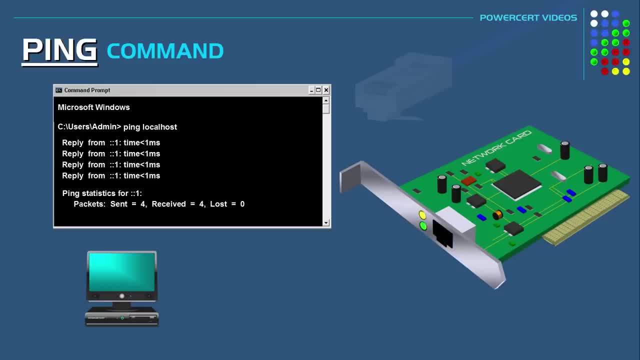 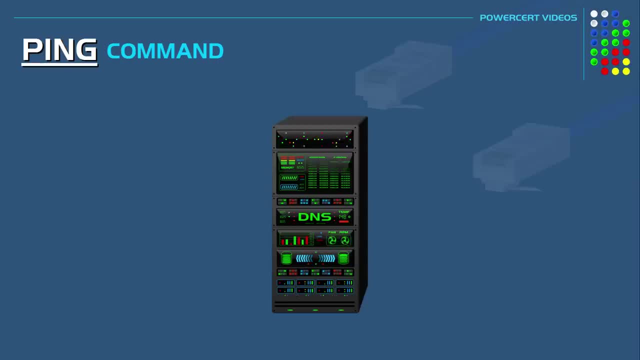 successful, then you can be assured that your network card is working properly. But if the loopback test, then there's a problem with your network card. Now the ping command can also be used to test DNS name resolution issues, And if you're not familiar with what dns does, please watch. 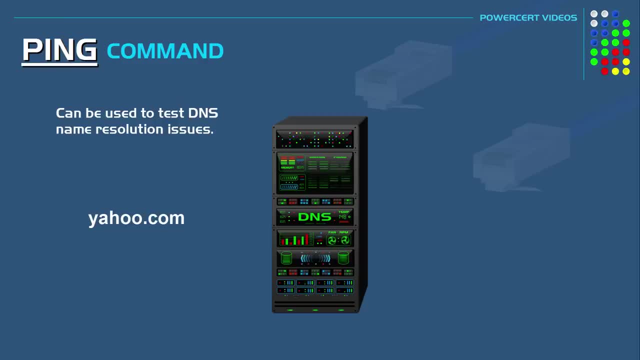 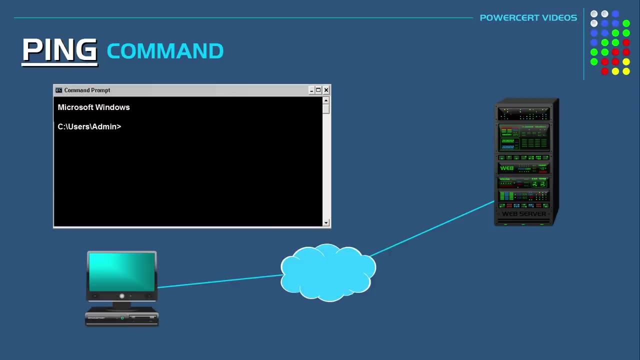 my DNS video on my youtube channel. But, in a nutshell, DNS is what resolves domain names to IP addresses. So, as you recall, earlier I did a ping test by pinging the domain name yahoocom instead of its IP address And, as I said before, if the ping looks different, thenviamente. 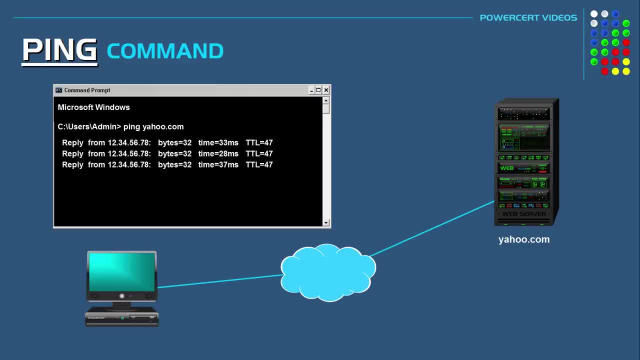 the ping was successful, then that means that all of my hardware is working correctly. But in addition, it also verifies that DNS is working correctly. So, as you can see, DNS successfully resolved and found the IP address for yahoocom. But if we pinged yahoocom and we got a message,